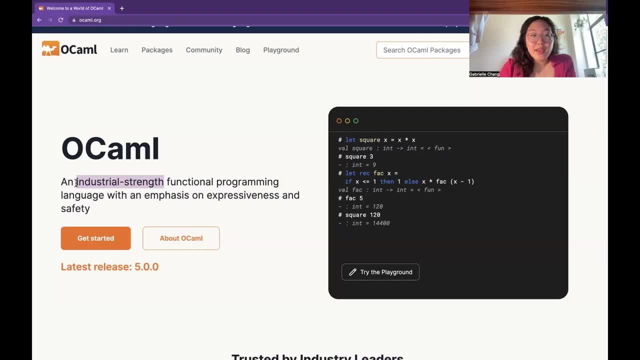 Jane Street in the finance industry to develop trading systems. Expressiveness: that means that you can write really concise code for really complicated stuff, which we'll see later. And safety is another really big feature of OCaml. It's known for its strong type system. 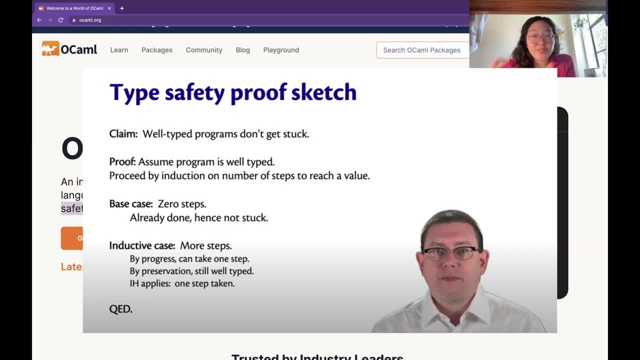 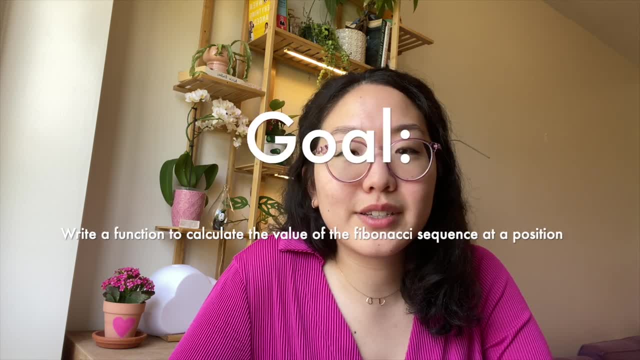 which means that it catches errors at compile time, before the code is even run. So that was a lot. I think a demo is the best way to see the stuff in action. So let's write a function that calculates the value of the Fibonacci sequence at a given position. 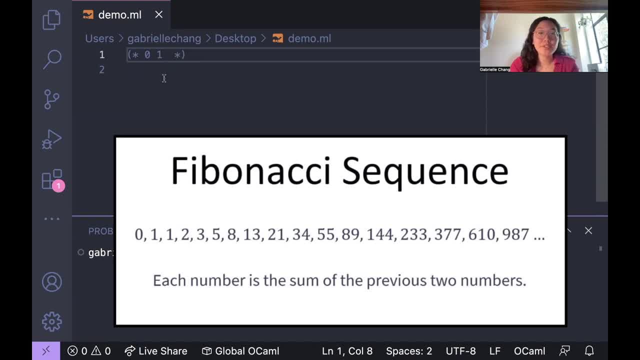 Okay, recall that the Fibonacci sequence is a series of numbers where each number is obtained by adding the two numbers that are immediately before it, starting with 0 and 1.. Those two added together are 1. 1 plus 1. added together is 2. 1 plus 2. 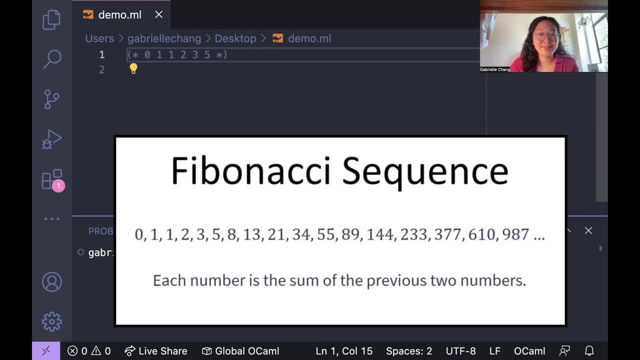 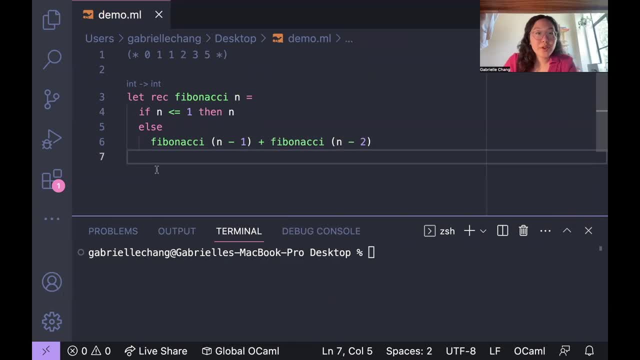 added together is 3.. 2 plus 3 added together is 5, and so on and so forth. So I'll go ahead and write the code now. So in this code we define a function called Fibonacci that takes in an integer. 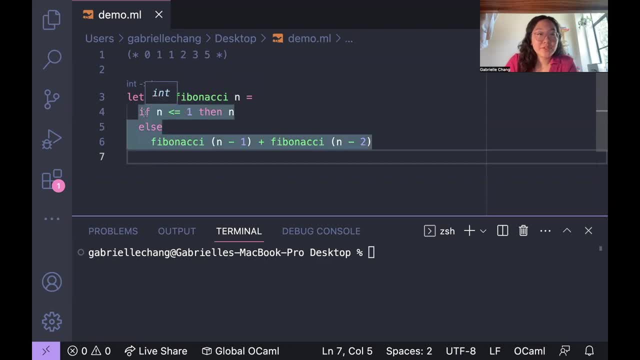 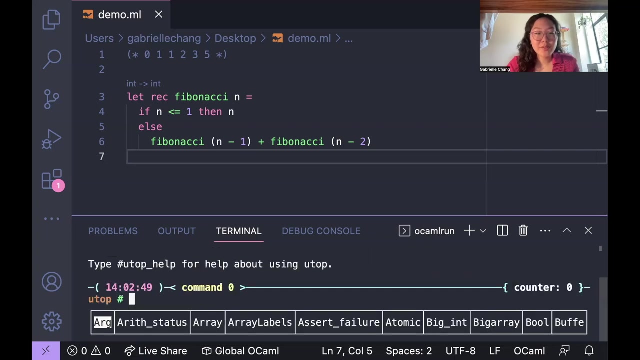 n as an input. So the function uses an if statement to check if n is less than or equal to 1.. And if it is, we return n, And otherwise we recursively call the Fibonacci function with n minus 1 and n minus 2 as arguments and add the results. Okay, to check that it's running properly. 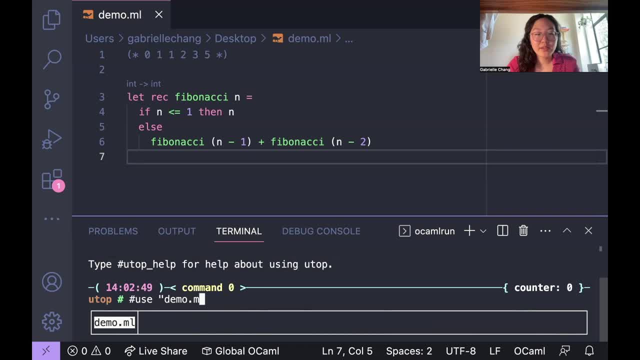 we can go ahead and try it. I'm trying it with 8, and it looks like it returned the correct answer of 21.. Very good, What if I told you that there's a more OCaml-y version to write this code? 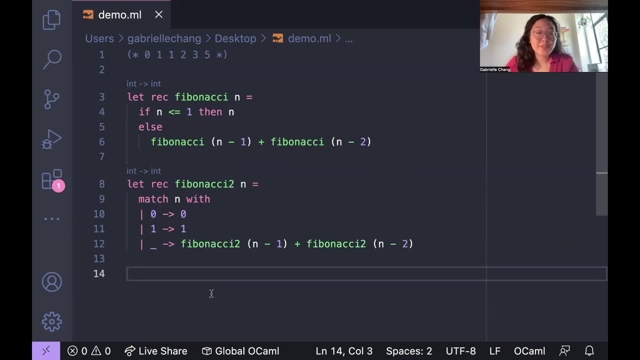 Okay, so we've written a second version of Fibonacci, and you'll notice that it has no if statements, but rather this sort of matching. So if statements are used in OCaml, but they're not as prevalent as they are in imperative programming languages. What's going on here? 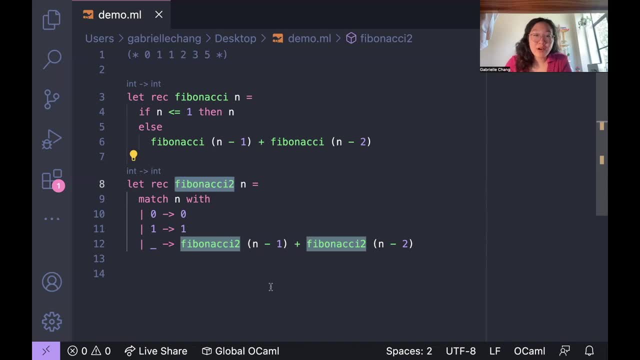 instead is pattern matching, which is this language construct often used in place of if statements, which allows developers to match values against patterns and execute code based on the match. So what's going on here is that we're passing in n and then the function asks: is n 0?? If so, return 0.. 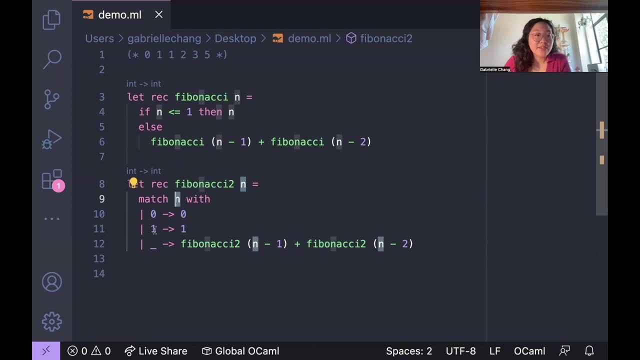 And then the function asks: is n 0?? If so, return 0.. And then the function asks: is n 0?? If so, return 0.. Otherwise, if n is 1, return 1.. And if n is anything else, what we're going to do is recursively. 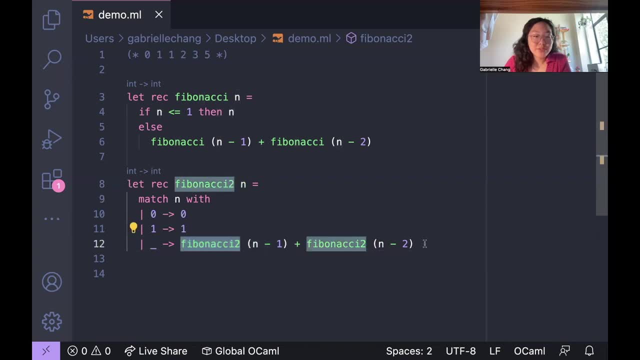 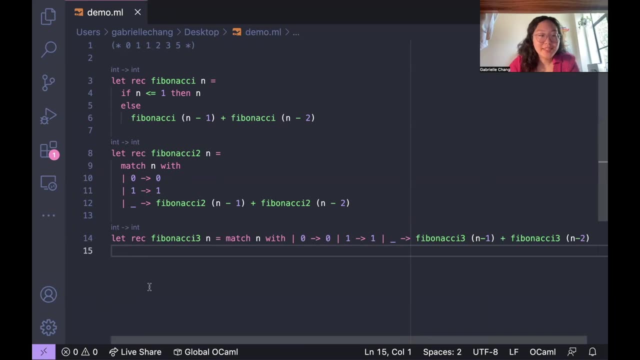 call the function again, passing in n-1 and n-2 as arguments and adding the result. For a little bonus, here's another way to write it. Okay, so this is a totally valid and correct implementation. You'll notice that it's basically. 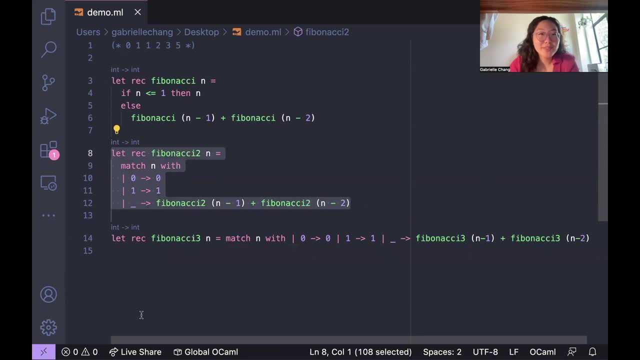 the previous implementation just in one line instead of multiple And honestly to me it's a little bit harder to understand compared to the previous version. But I just wanted to include this because functions in OCaml are often written in a very super concise and compact style. 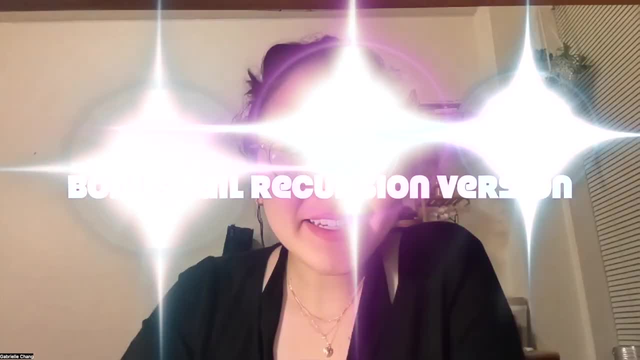 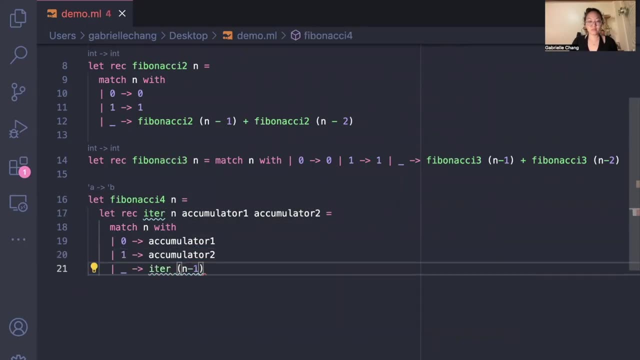 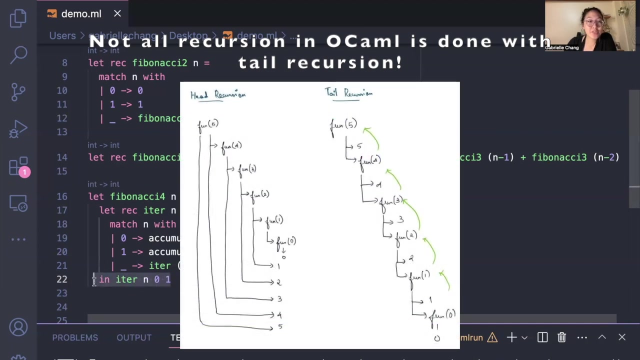 and sometimes this means that there's a lot being fit on a single line. While editing this video, I got a bit carried away and I want to show one more version to rewrite this function. Recursion is found in many programming languages, but OCaml uses tail recursion, which is a type 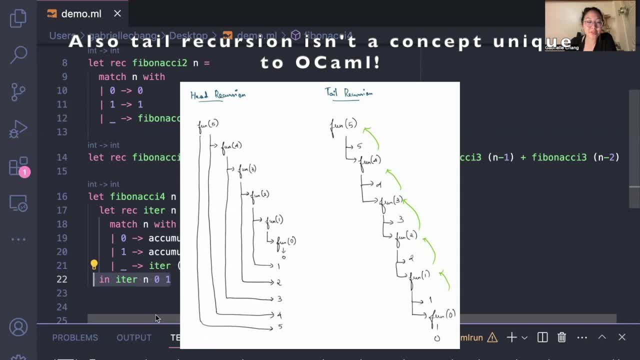 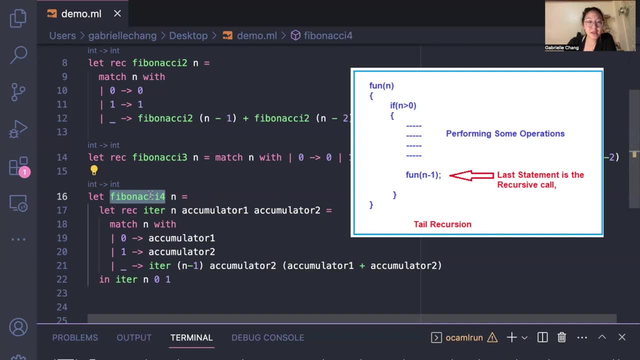 of recursion in which the recursive call is the last operation in the function. So a common pattern. functional programming is a main function which takes in the arguments needed to calculate the final output and a helper function to perform the actual recursive computation, which is iter in our 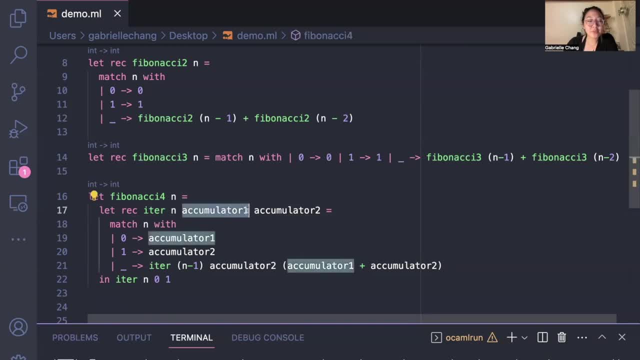 case. What's different here is we have two accumulators called accumulator 1 and accumulator 2, which store the last two Fibonacci numbers. As before, we basically add up the last two Fibonacci numbers and you'll notice right here that we call the helper function and we pass in the position. 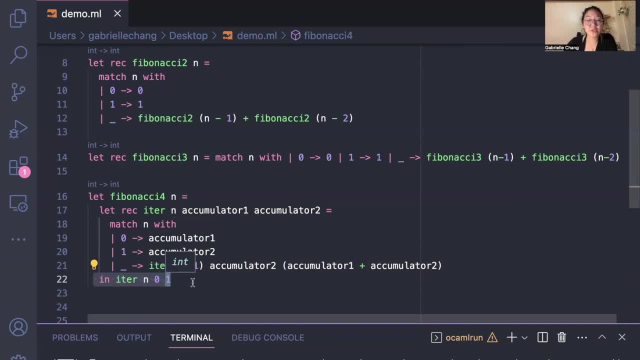 that we're looking for, as well as 0 and 1 to represent the first two Fibonacci numbers in the sequence. So the whole point of having this helper function and doing everything tail recursively is that it allows the compiler to optimize the code by reusing the same stack frame for each recursive. 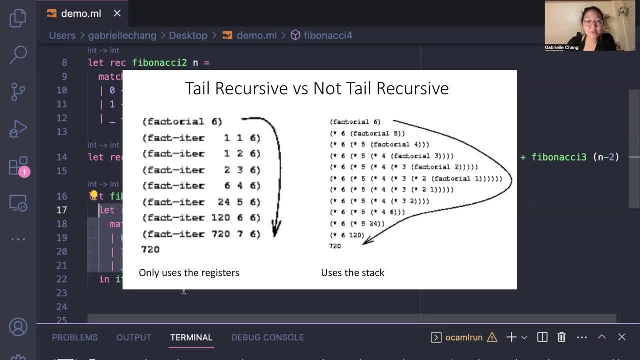 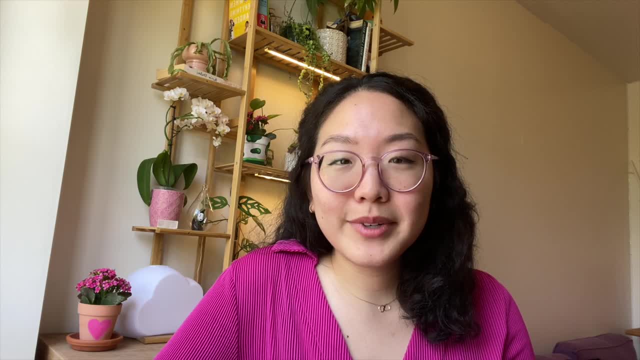 call rather than allocating a new stack frame for each call, and this overall just prevents stack overflow errors if we have a really really large N. So yeah, that was a taste of this very distinct style of programming with OCaml. If, by the end of this video, you're like that's cool, but I'm 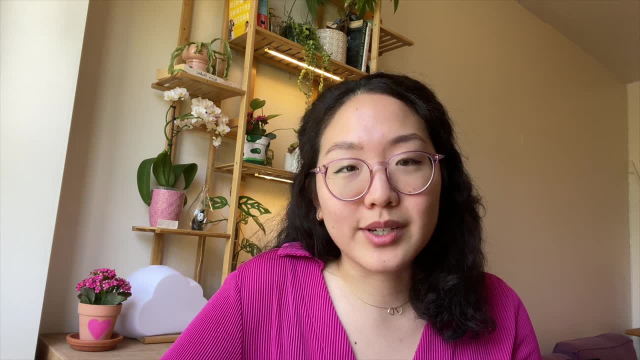 probably not going to use this. That's okay. I always encourage you to explore what resonates with you and your interests, whether it's a specific language like OCaml, or whatever. Subscribe for more videos.